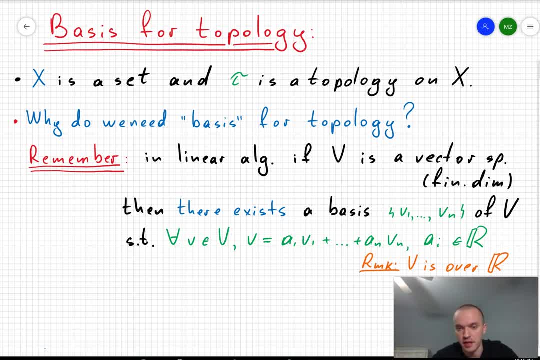 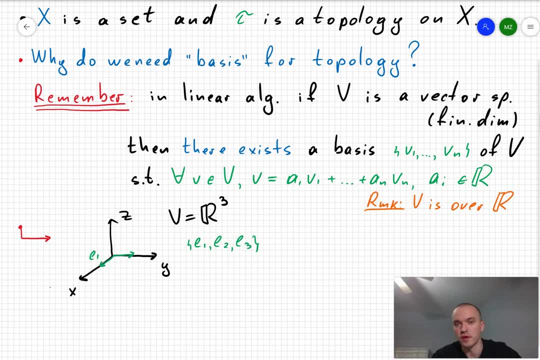 as a linear combination of real coefficients of the basis elements. For example, let's take a three-dimensional vector space. Then in this case I can choose a basis to be unit vectors, along like X, Y and Z direction, And those vectors are going to generate our 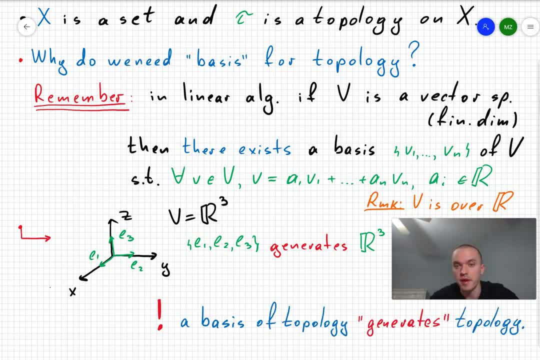 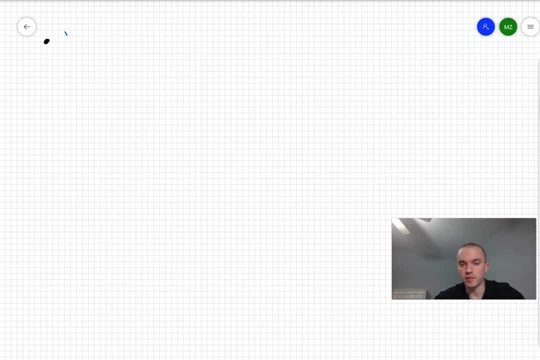 three And the same for basis for topology. A basis for topology- I'm going to explain it later- is going to generate our topology. So what is a basis for topology? To define a basis for topology, what do we need to do? We need to take some set X and 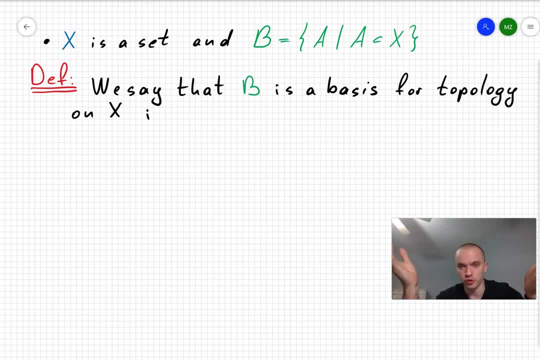 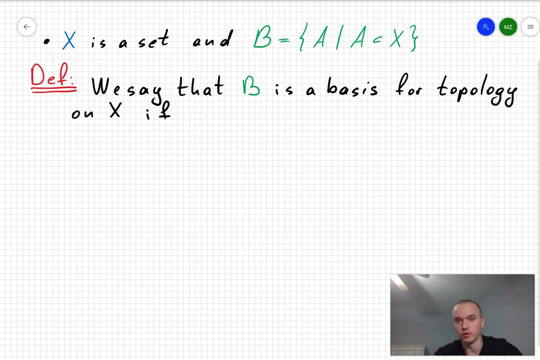 some collection of subsets which we're going to call V, And then we're going to say that V is a basis for topology on X, if two conditions are going to follow. So first condition is some sort of existence, If we want to take any element in our set. 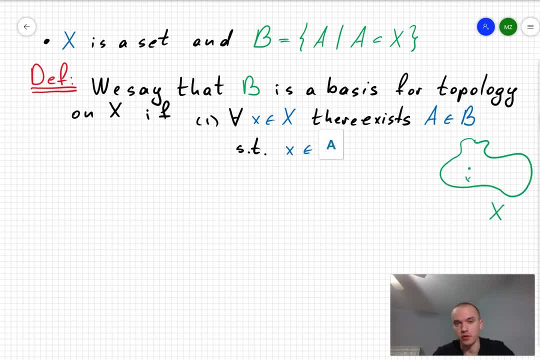 X. we always want to find some element A in our base, so like some subset of X, such that our element X is a basis for topology, The place where us element X is going to belong to the subset, When, as I say, you can see in: 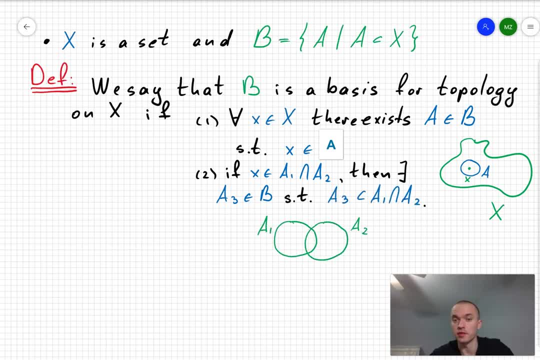 this picture. we just want to find some open bowl around your point X. The second assumption is really in wound. to take any two elements of your basis, A1 and A2, intersect them And then your intersection's then empty. then for every element inside. 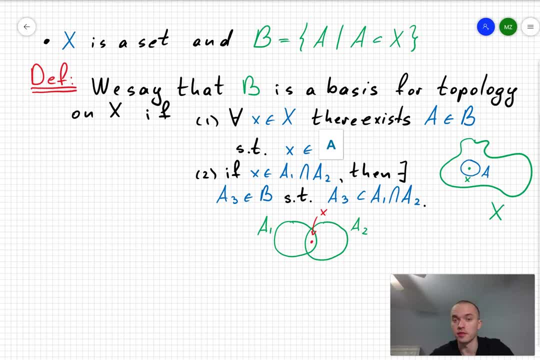 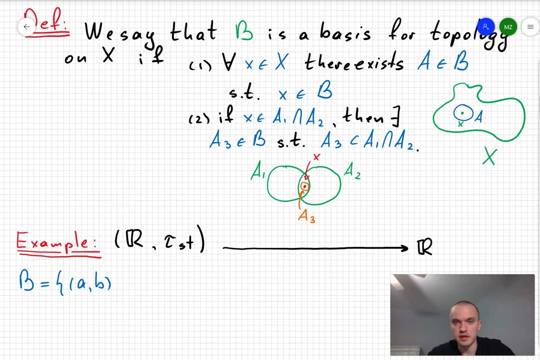 you intersection, you always must have some other element A3 of your base, Since that only is subset of A1, intersection A2.. Let's do some example. Consider like a real line in the standard topology, and I'm going to define B as a union of open intervals, AB. I want to show that B is a. 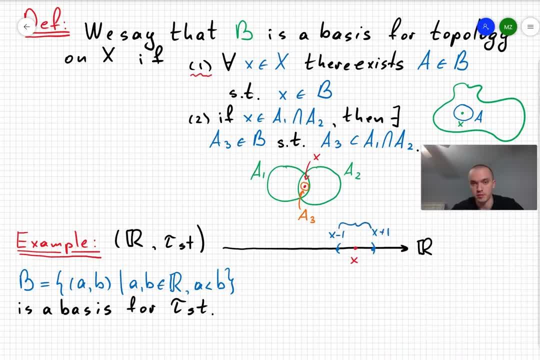 basis for our standard topology. For that I need to check the first and second assumption. For the first assumption, take some x on your real line and if you're going to go one to the left or one to the right, you're going to obtain an open interval: x minus 1, x plus 1 and that open interval obviously. 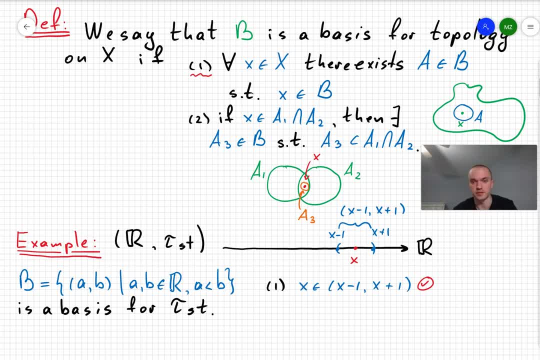 belongs to B. So that's why the first assumption satisfies. To show the second assumptions we need to take some two elements of our like basis. then those two open intervals are going to be either intersect or not. If they're going to intersect, then you can see that intersection of AB and CD.